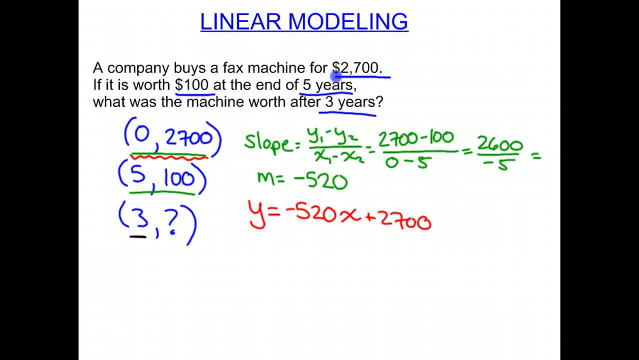 And then we need to find out, when x is 3,, what will y be? So y equals negative 520.. x is 3 plus $2,700.. So then we multiply: y equals negative 1560 plus $2,700. 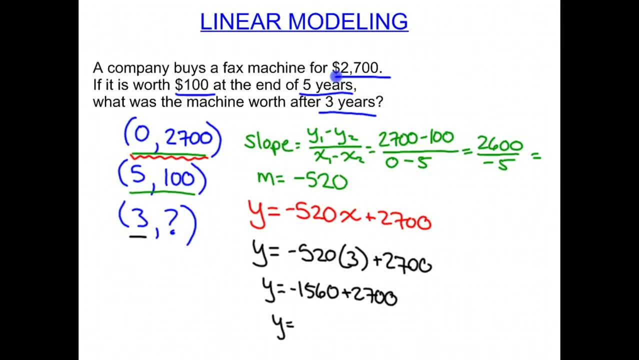 We simplify this and we get $11,040.. So our answer: when x is 3, y will be $1,140.. That's our answer And remember it's in dollars because it is an amount. So what was the machine worth after three years? 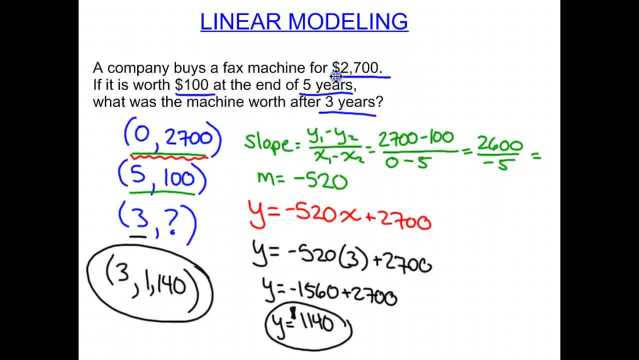 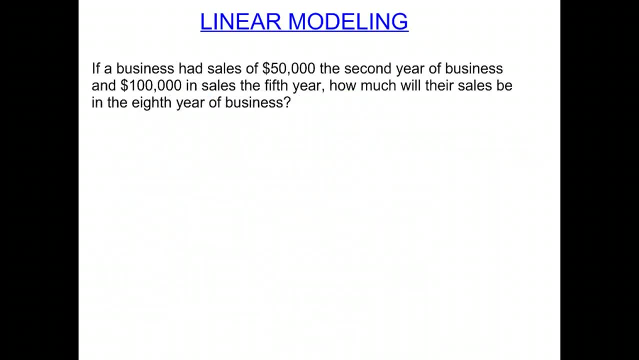 The machine was worth $1,140.. Let's look at another example. If a business had sales of $50,000 the second year of business and $100,000 in sales the fifth year, how much will their sales be in the eighth year of business? 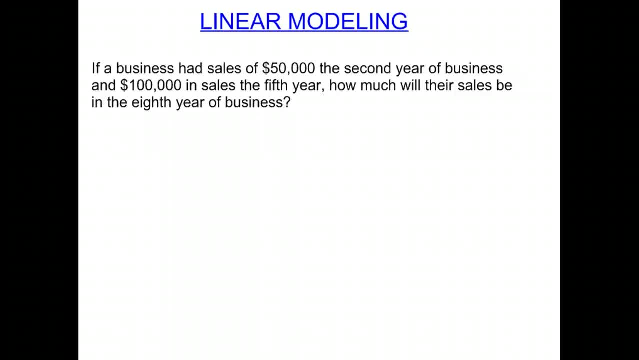 So again, we're going to look at those points. So they had a sale of $50,000 in the second year. So remember, the sales depends on the year. So we have second year was $50,000.. And then we have sales of $50,000. 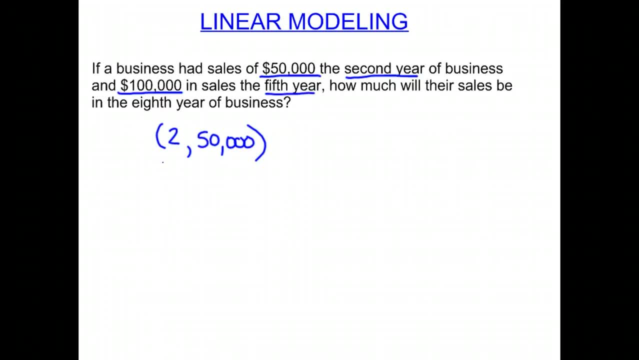 And then we have sales of $100,000 in the fifth year. So five years they do $100,000.. How much will their sales be in the eighth year of business? So in eight years, how much will they make? Again, we can find our slope by using the first two points. 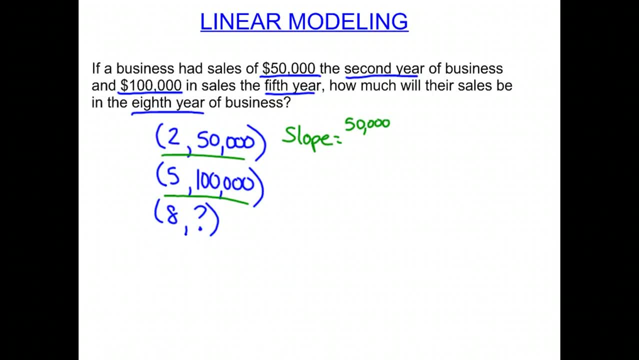 So we do our y: $50,000, minus $100,000.. $100,000 divided by 2 minus 5, which is negative. $50,000 divided by negative 3. Negative cancel. So our slope is $50,000 divided by 3.. 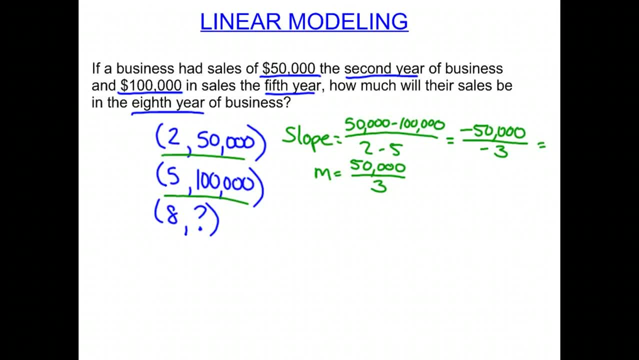 Now we don't have our y-intercept this time, So we're going to have to use point-slope form. So we say y-minus. we'll use this first equation for the point. So y-minus 50,000 equals our slope $50,000 divided by 3, times x-minus 2.. 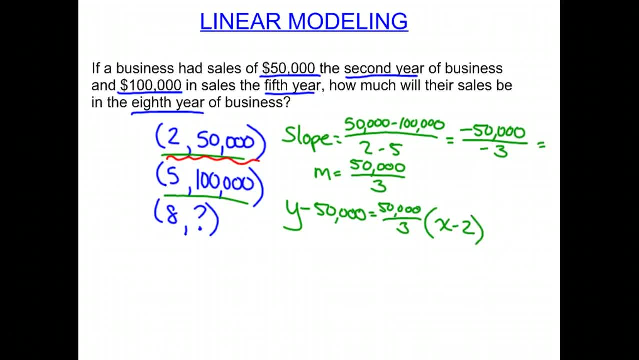 Remember, we're using those point values And we have to find out When x is 8,, what will y be. So y minus 50,000 equals 50,000 over 3 times 8 minus 2.. 8 minus 2 is 6, so y minus 50,000 equals 50,000 divided by 3,. 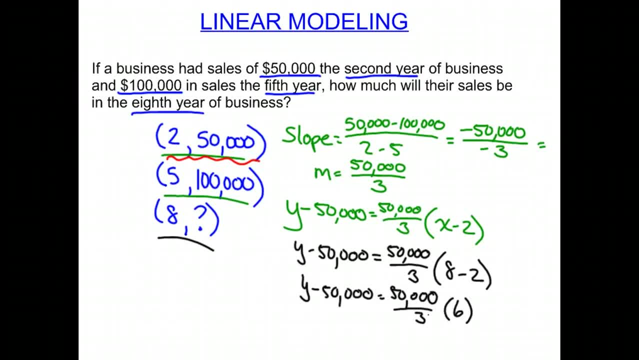 and we'll be multiplying by 6.. Now the 3 and the 6 can simplify or reduce. That becomes a 2. So y minus 50,000 equals 50,000 times 2,, which is 100,000.. 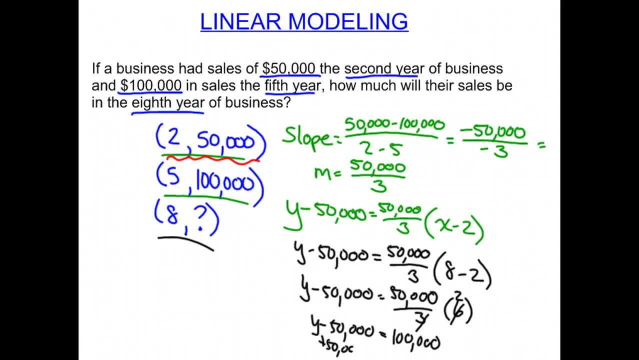 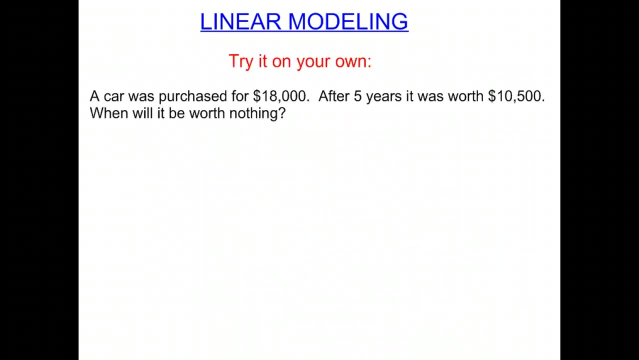 And then we just have to add our 50,000.. So we get: y equals 150,000.. Okay, and that is our answer for the 8th year of business. So what I'd like you to do is try one on your own. 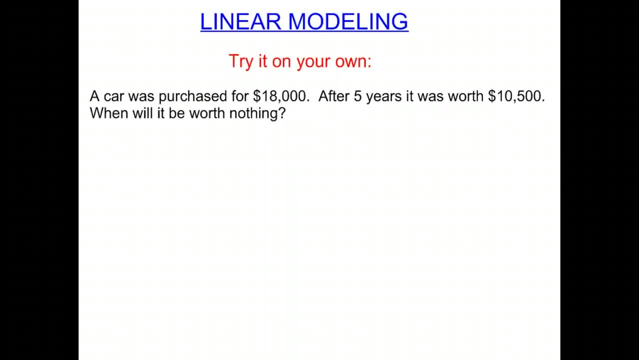 So a car was purchased for $18,000.. After 5 years it was worth $10,500.. When will it be worth nothing? So remember you need to find your points first. So look at the information and get your two points. 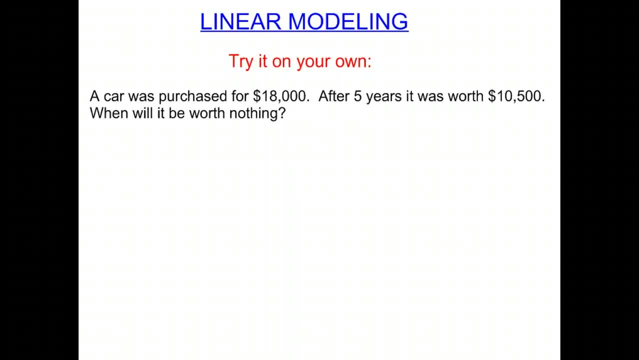 Then try to find out what you're trying to find. Are you looking for the x? Are you looking for the y? What information do you have? Find the equation to use. Okay, make sure you find your slope, then find the equation. 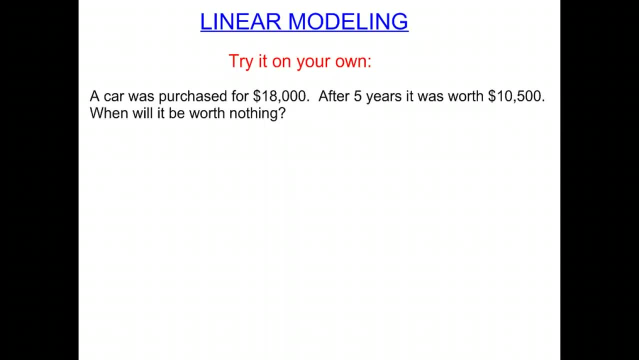 And then you can solve for what you're looking for. Good luck.